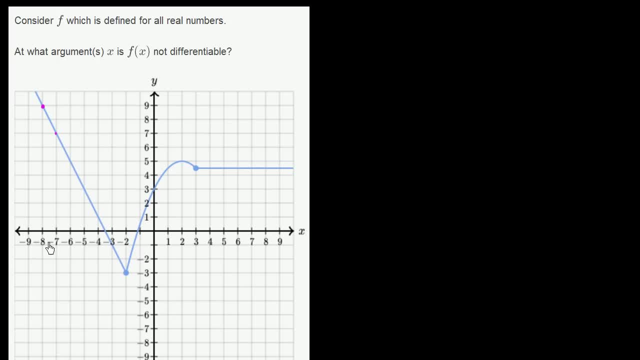 It looks like the slope is a constant negative 2.. So if I were to draw its derivative, its derivative would look something like this: Its derivative looks something like this. But then something interesting happens at: x equals negative 2.. Right, as we cross, x equals negative 2,. 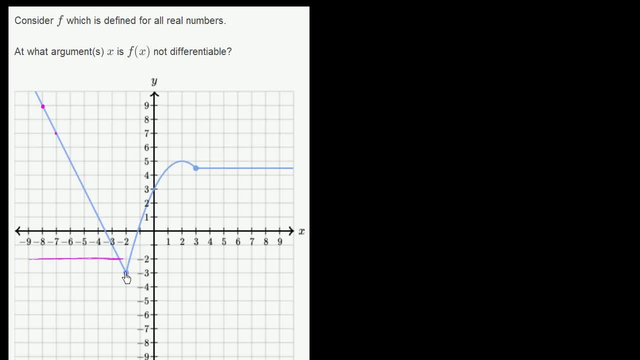 it looks like the slope goes from being negative 2,. it looks like the slope goes from being negative to being positive And it looks like right out the get go. if I were to estimate the slope of its tangent line, it starts changing. 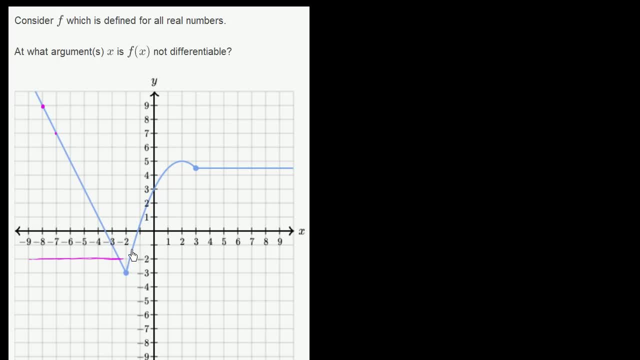 It's not a line anymore, It's a curve. The slope of the tangent line right at this point looks like it's around 3 and 1 half, Because if I were to draw its tangent line right over here, it looks like if I move 1 in the x direction. 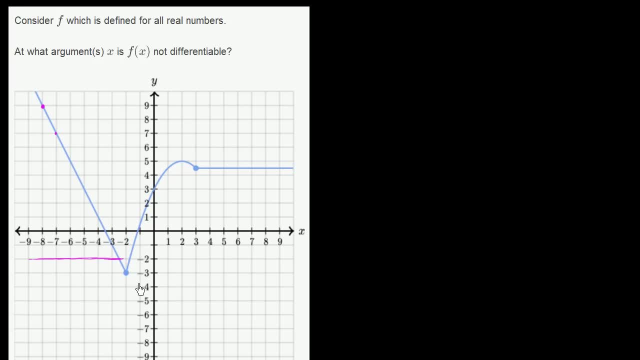 I move up about 3 and 1 half in the y direction. So I'm just trying to obviously estimate it. So it looks like the slope goes up to 3 and 1 half right when I cross that point, And then the slope becomes lower and lower and lower. 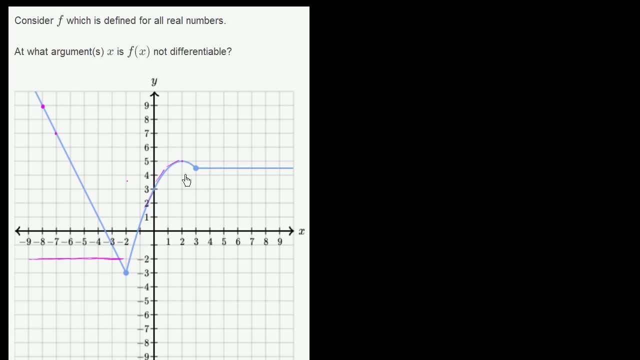 all the way until I get to this point right over here, all the way until I get to x equals 2.. And it looks like it continues to get lower all the way until you get to x equals 3.. So it looks like the slope of the line is getting lower. 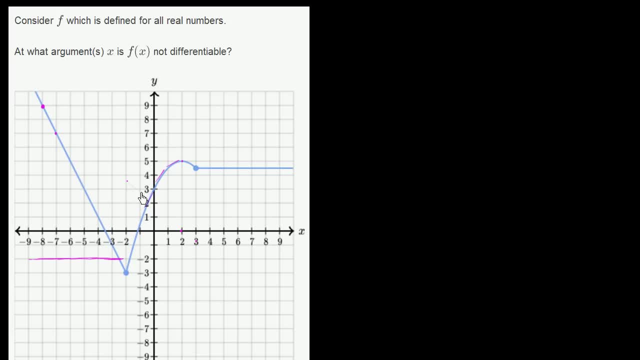 at a constant rate. I guess I could say So. it looks like it's doing something like this, Something like this, over this interval. But then, right as x crosses 3, this becomes a flat line. The slope is 0 here. 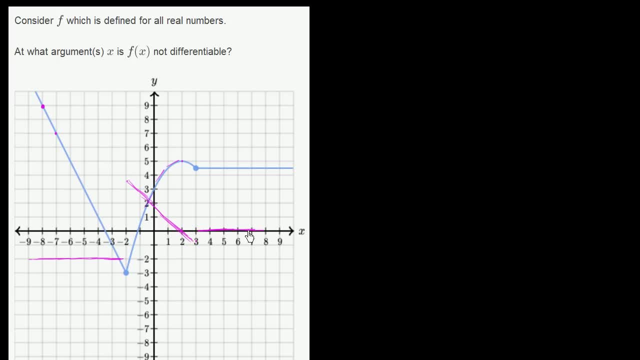 So right, as x crosses 3, the slope becomes 0. So we immediately see, there are points where it looks like the slope jumps, And at these points we really don't have a defined derivative. The slope jumps there as well. And so at what arguments is f not differentiable? 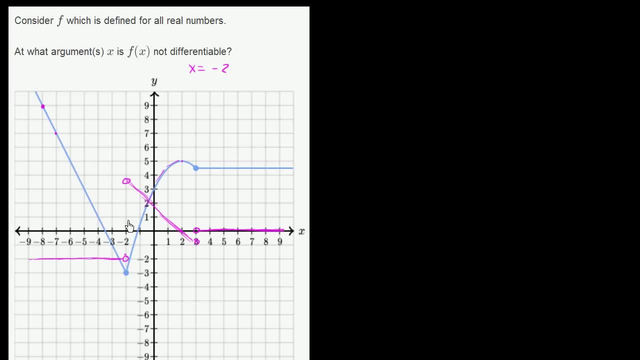 Well, it's not differentiable when x is equal to negative 2.. We really don't have a slope there. Remember, when we're trying to find the slope of the tangent line, we take the limit of the slope of the secant line between that point.